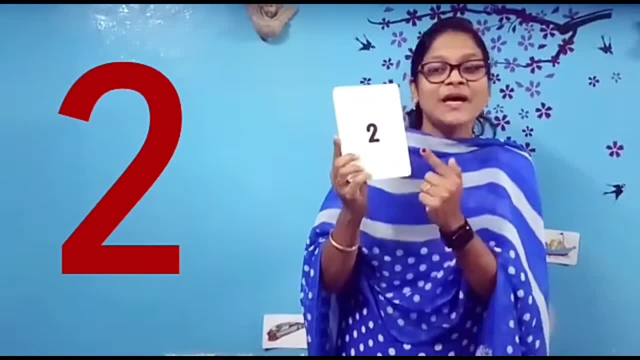 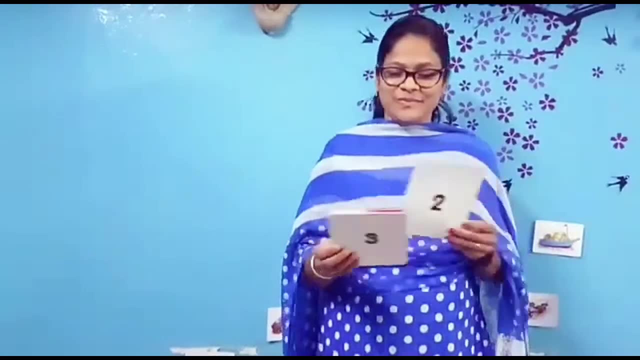 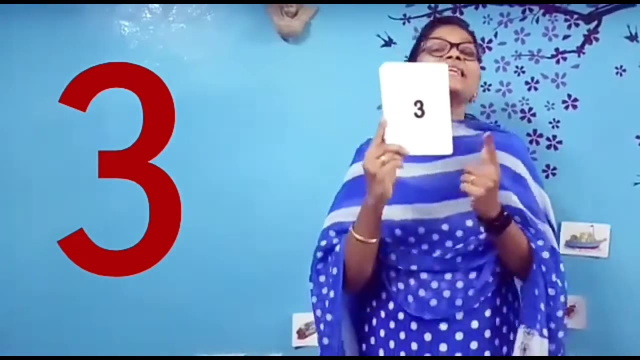 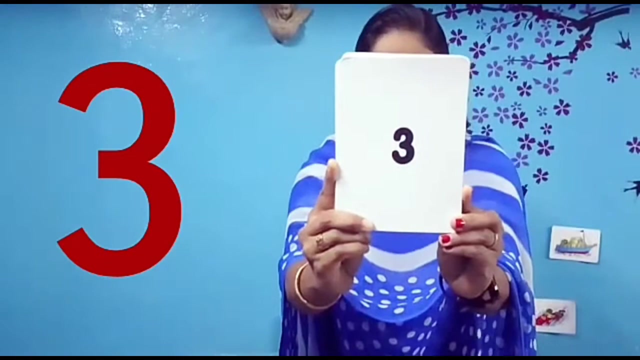 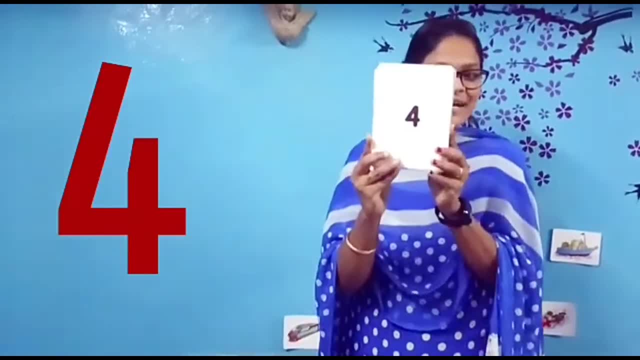 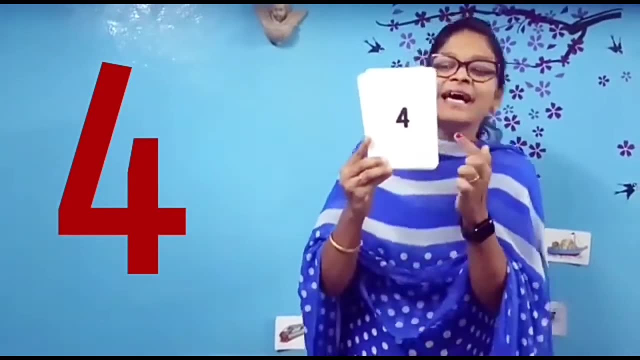 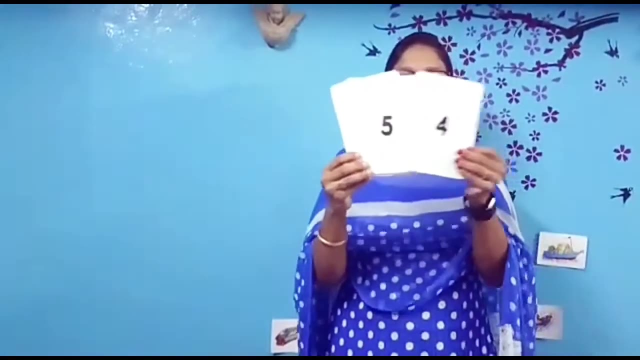 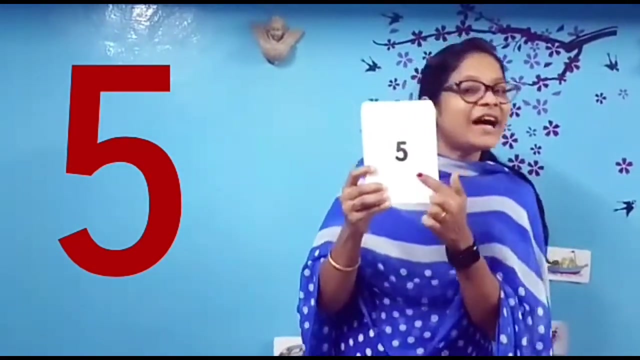 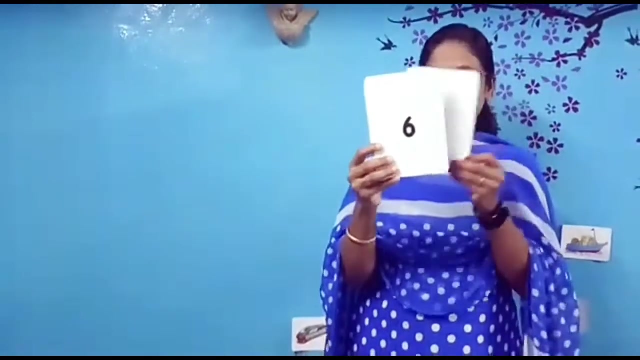 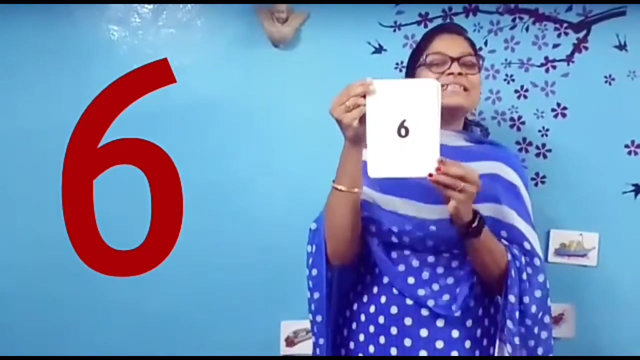 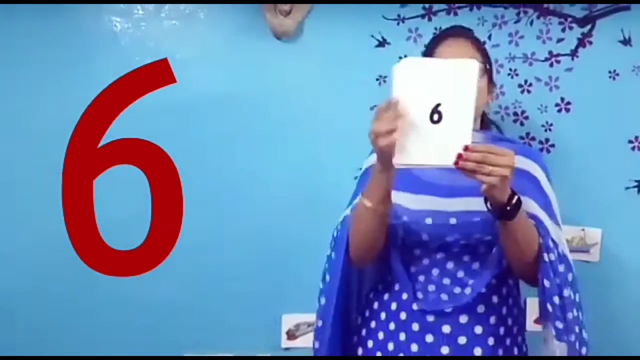 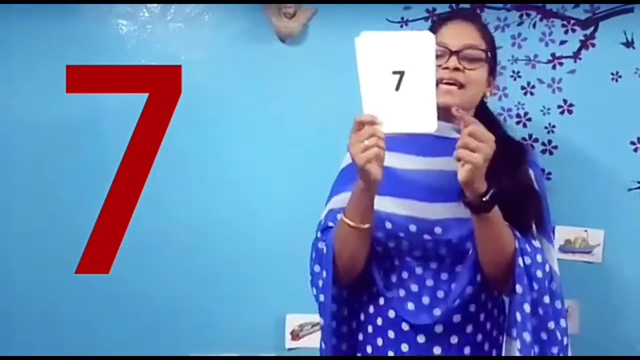 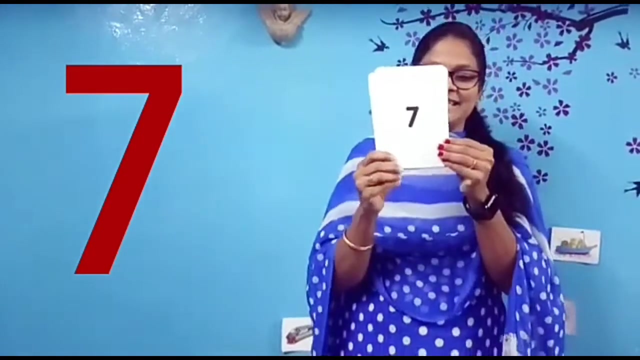 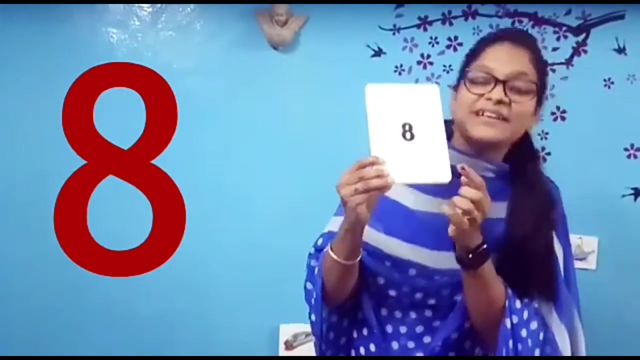 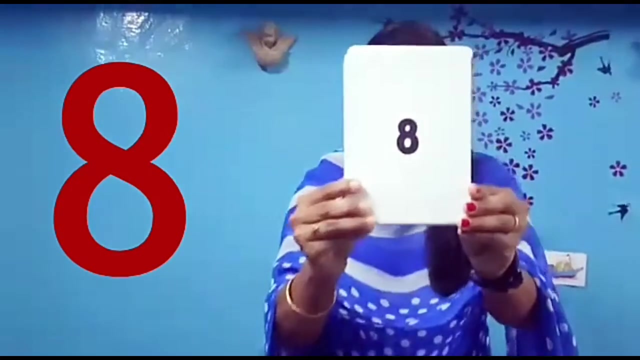 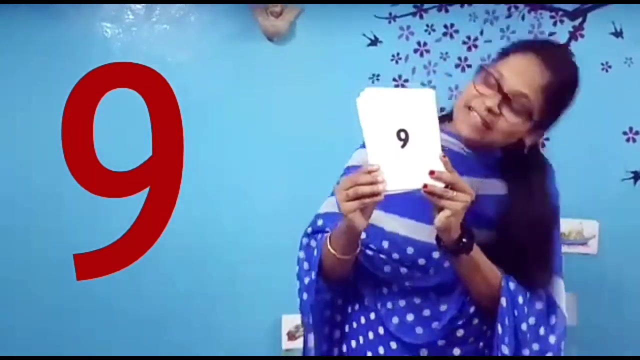 the next number four: number four, number four. this is number four. five: number five: number five. this is number five. very good, now tell me number six, number six. this is number six. seven: number seven: number seven. this is number seven. the next number eight: number eight: number eight. this is number eight. number nine: number nine. 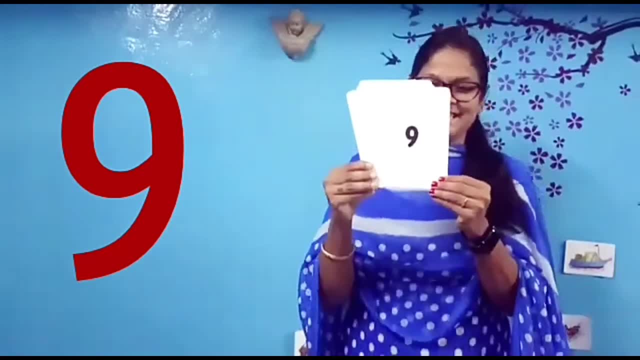 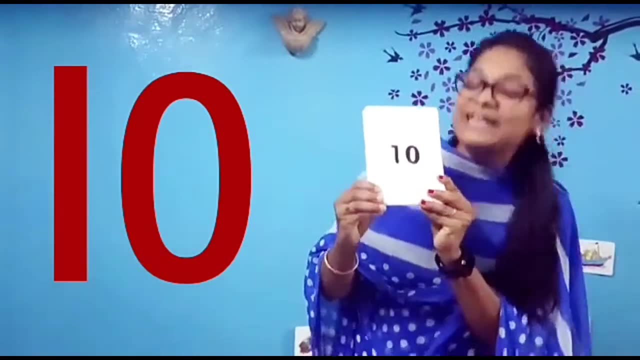 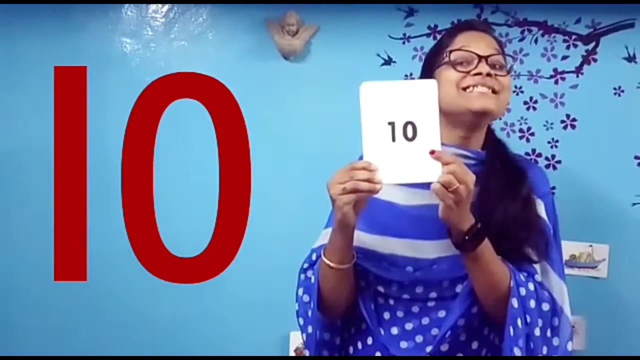 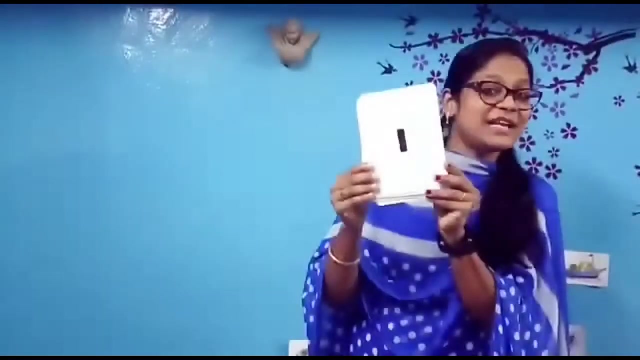 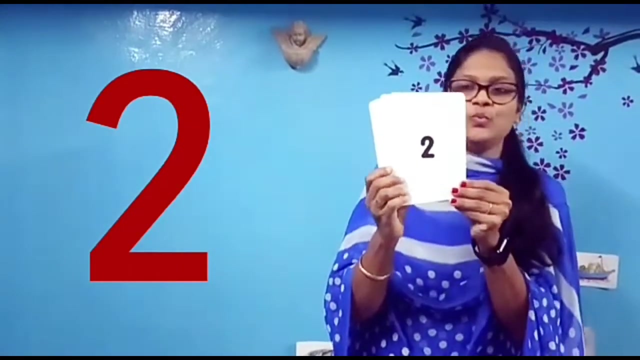 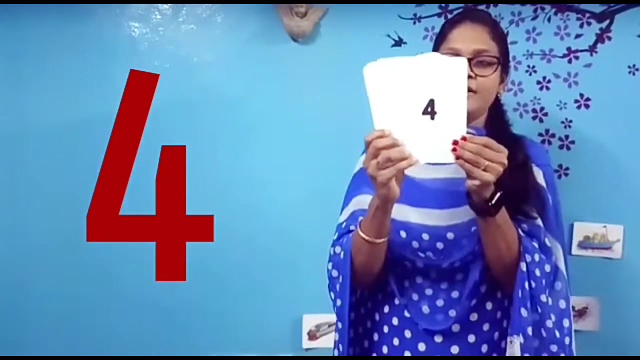 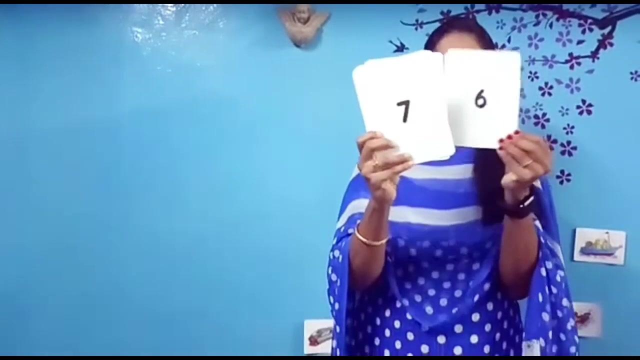 is number 9, number 10, number 10, number 10. this is number 10. very good, now let's see once again. tell me fast: 1, all of you say 1, 2, 3, 4, 5, 6, 7, 8. 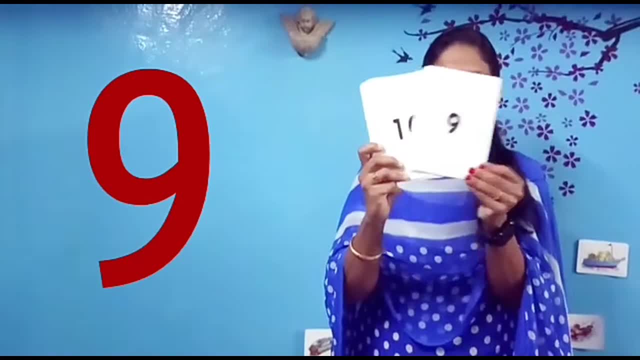 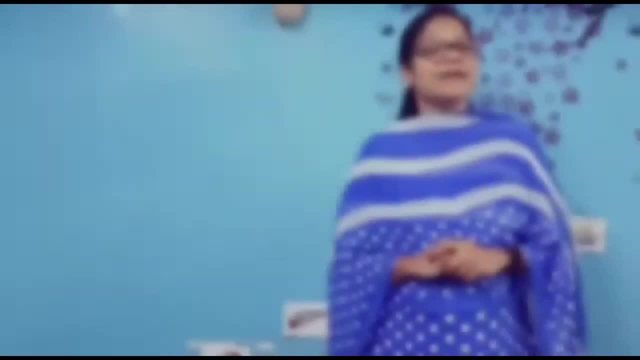 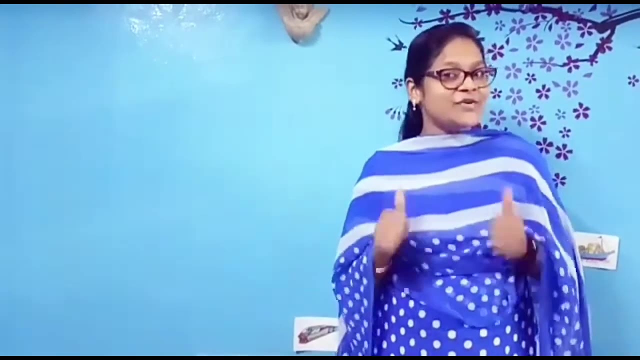 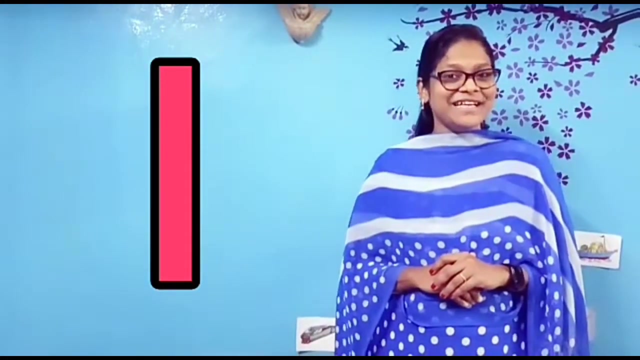 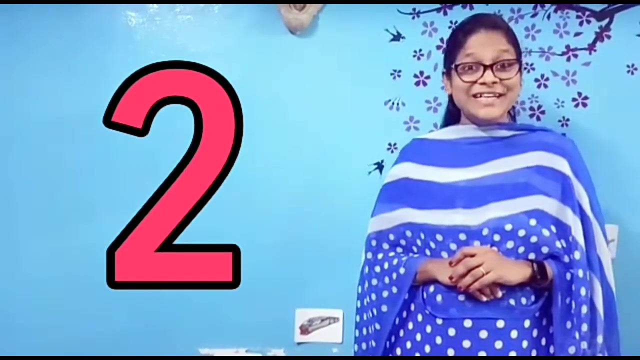 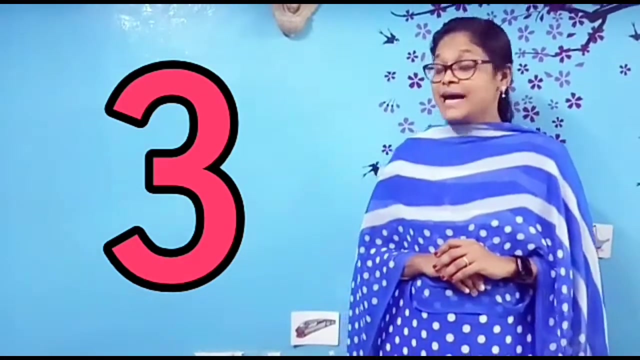 9, 10. very good. now, my dear students, you try to say the numbers as it is displayed. are you ready? get ready. tell me what number is this? very good, it's number 1. now tell me what number is this? 0- Good, It's number 2.. Now tell me, what number is this? Number 3.. Good job, Now tell me what. 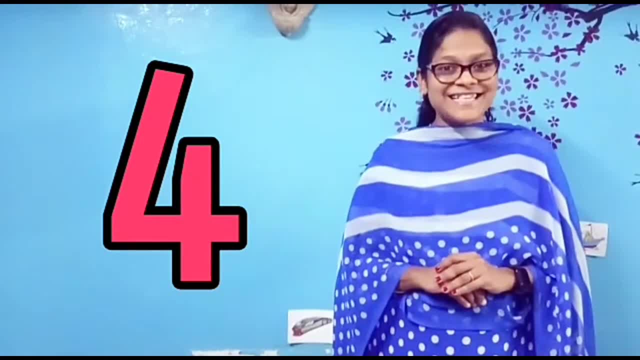 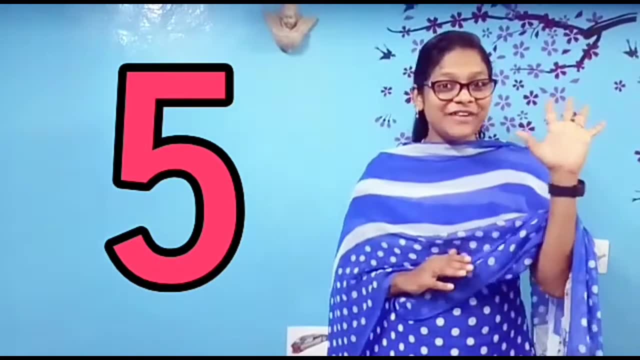 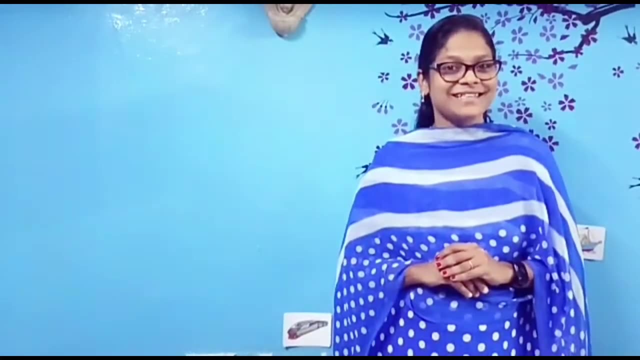 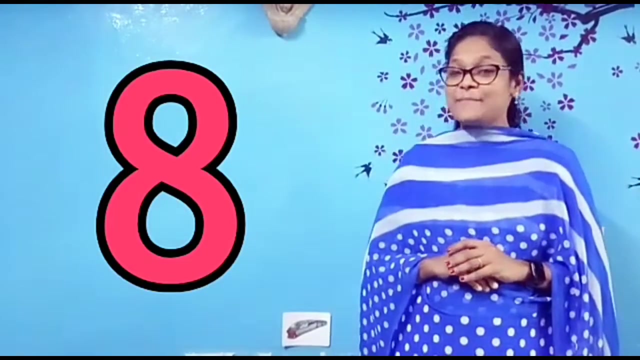 number is this: 4. Excellent. What's the next number? 5. Very good, The next number: 6.. What's the next number? 7. Tell me the next number. 8. Very good, Now tell me what. 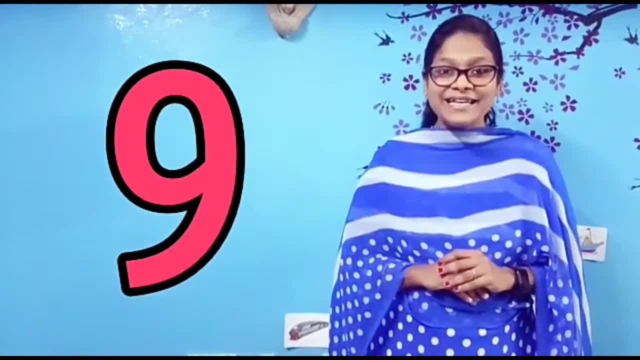 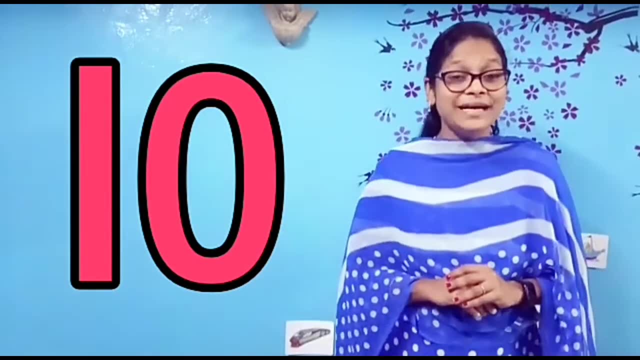 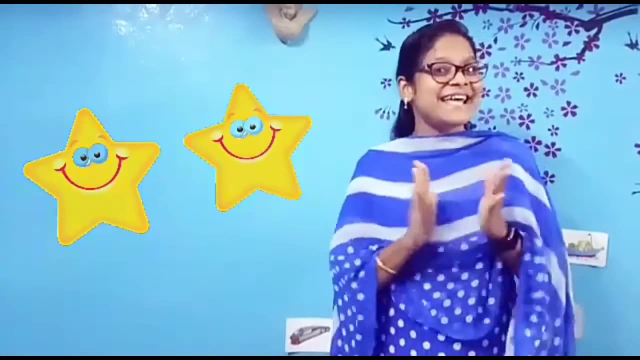 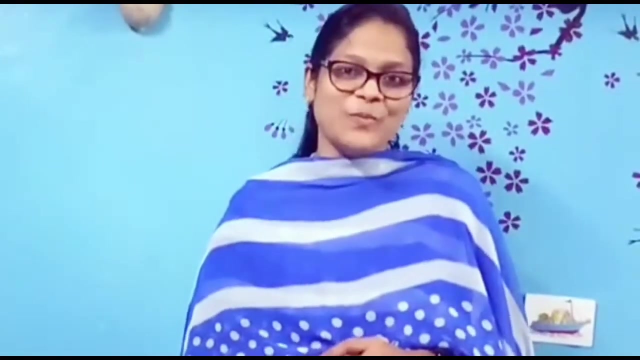 What number is this? Number 9.. What's the last number displayed over here? It's number 10.. Well done, Mom is giving you 2 stars. Excellent, Very good. All of you should practice the numbers 1 to 10 at home. Bye, bye, children. You spend $45 setting up your lemonade stand right. It costs you 10 cents in supplies to make each glass. You charge 75 cents for each glass. How many glasses of lemonade do you have to sell to break even? So there's this concept here of breaking even. Let's talk about that for a minute. 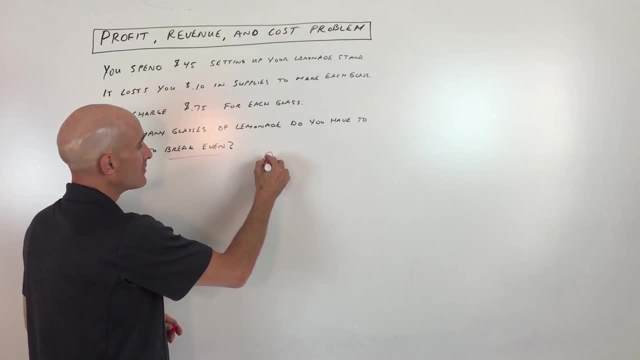 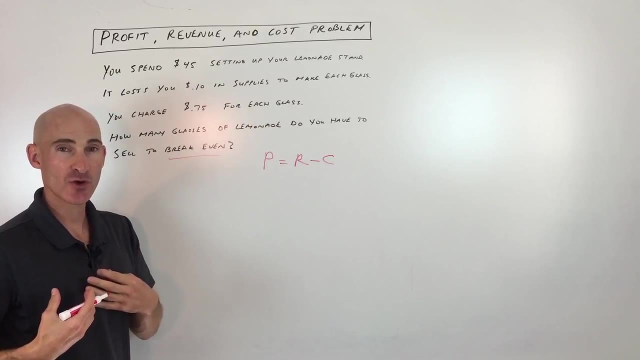 So when you look at these variables, you've got profit, which equals the revenue, how much you take in minus the cost. So revenue is what you take in, that's the amount of money you earn minus what you spend to buy supplies and to set up your stand and so forth. 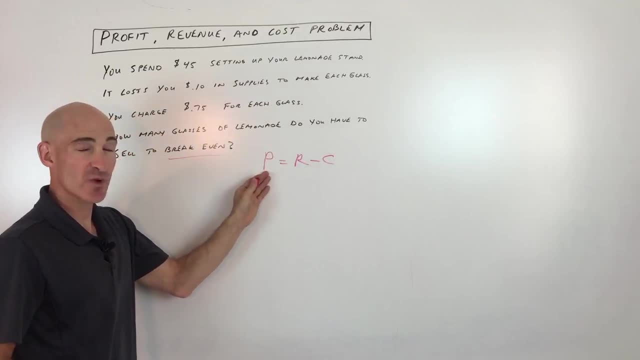 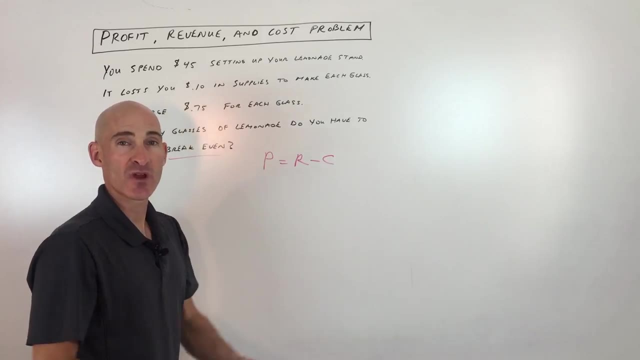 and you're left over with the profit. Now the break even point is just when you are about to reach the profitability. You've paid for all your initial costs and after that you're going to start becoming profitable. So that's when the profit equals zero. 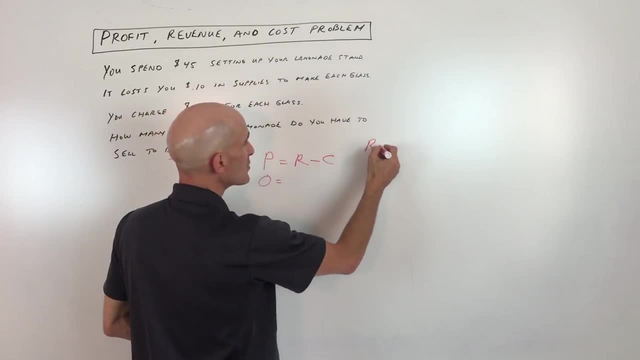 Okay, so let's write an equation for the revenue. So the revenue is what you take in, that's 75 cents times x the number of glasses of lemonade that you sell. Now the cost, let's see: you have an additional cost, you have an additional cost. you have an additional cost, you have an additional.